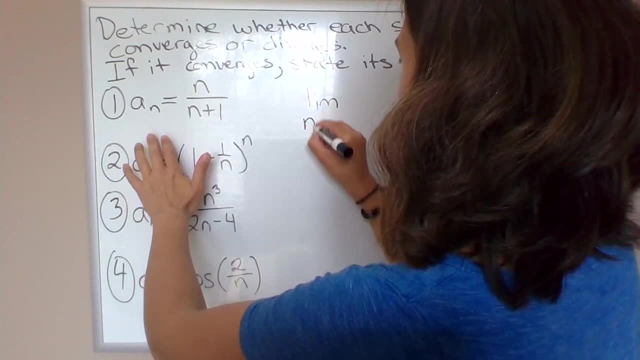 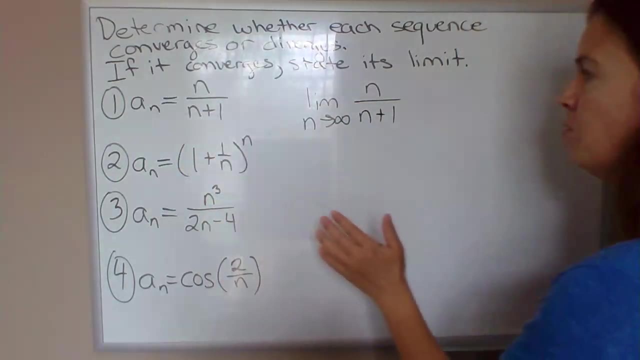 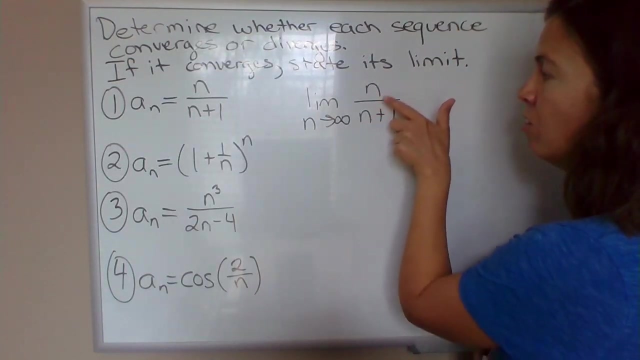 this first example. so we can determine whether this sequence converges or diverges by taking the limit as n approaches infinity of n over n plus 1.. Now, with this limit, the thing to notice is that I've got the rational expression with the same degree in the numerator and denominator, And 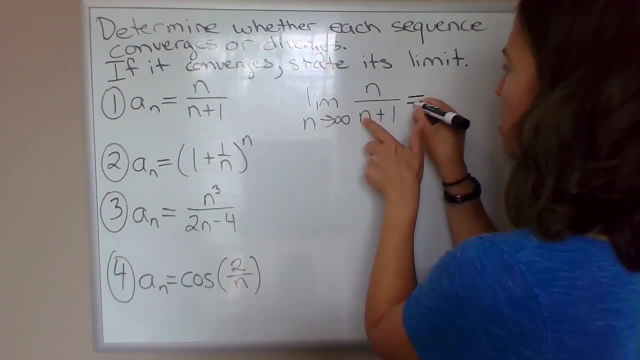 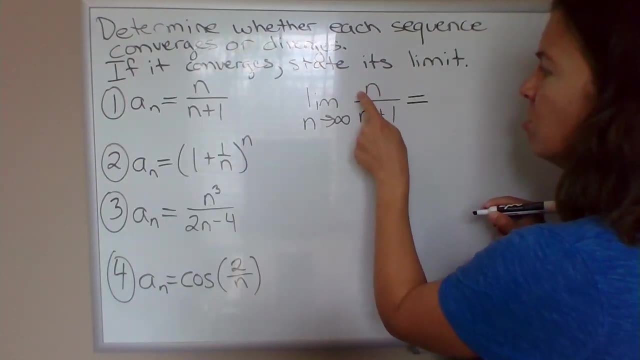 so when you have same degree in the numerator and denominator like this, the limit at positive or negative infinity is equal to the ratio of the leading coefficient, So in this case 1 over 1.. So the limit here is 1.. You could also use L'Hopital's rule. It's got the formant. 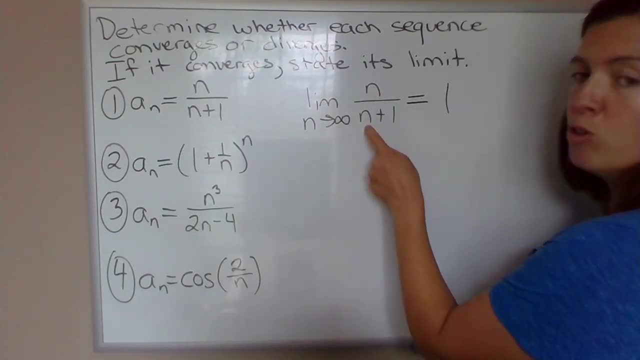 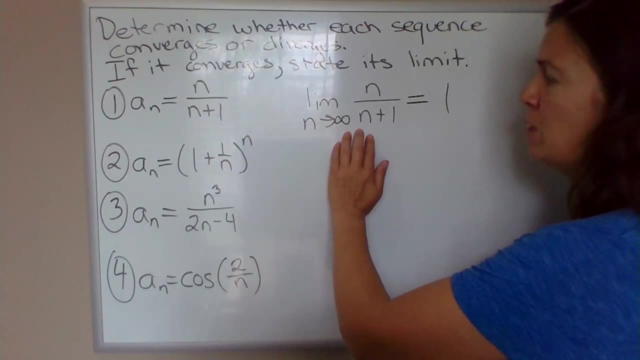 infinity over infinity. So you could take the derivative of the top and the derivative of the bottom, which would also give you 1 over 1.. But we're going to see limits of this form a lot, And so it's really best if you can recognize rational expression: same degree top and bottom. I just do. 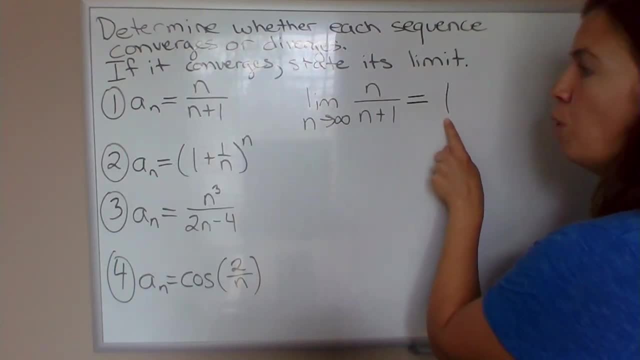 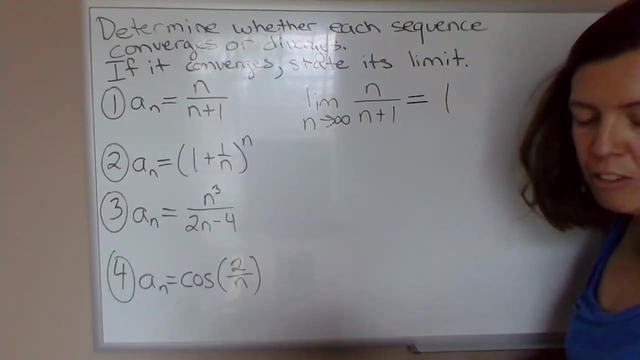 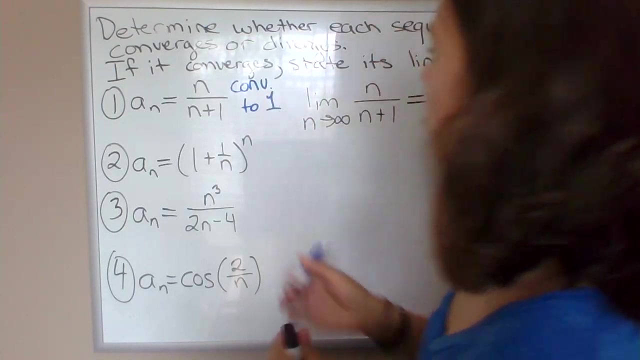 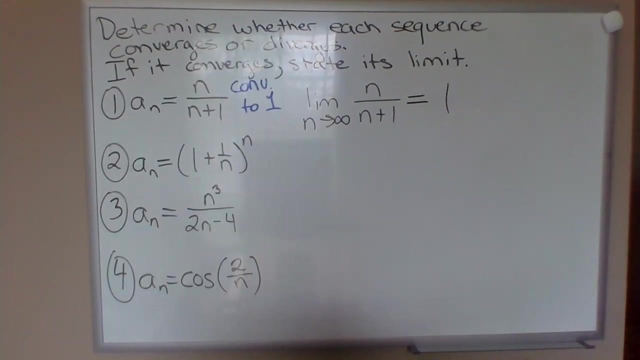 ratio of leading coefficients. It'll save you time. So when the limit is a finite number, as it is here, that means that the sequence converges to whatever that value is. So example 1 here converges to 1.. That's our answer, OK, And I'm going to erase. I won't erase yet, Actually I think I. 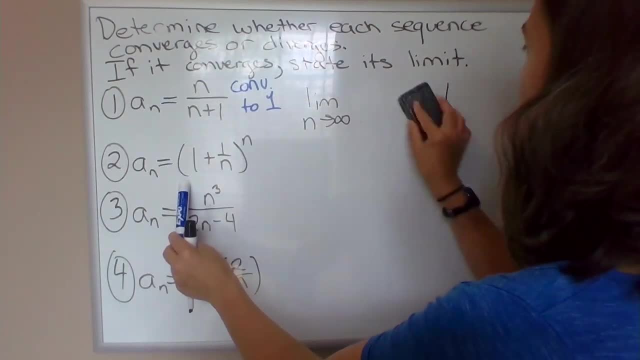 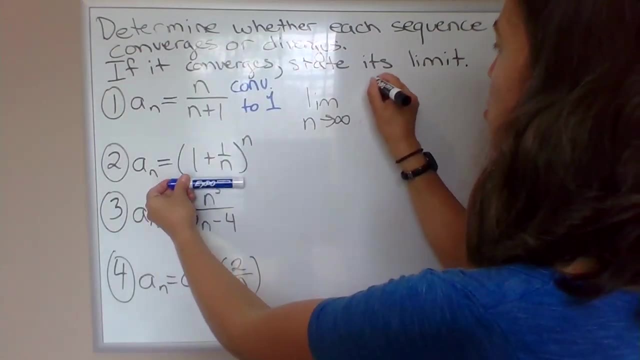 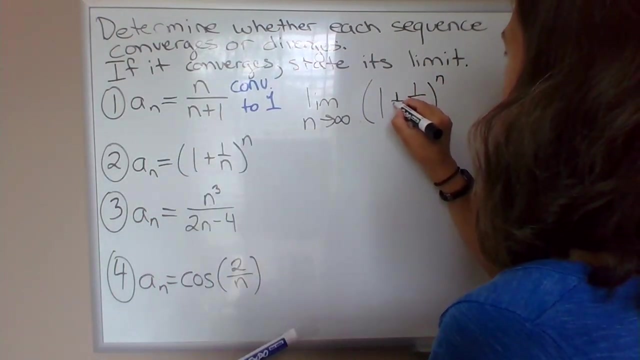 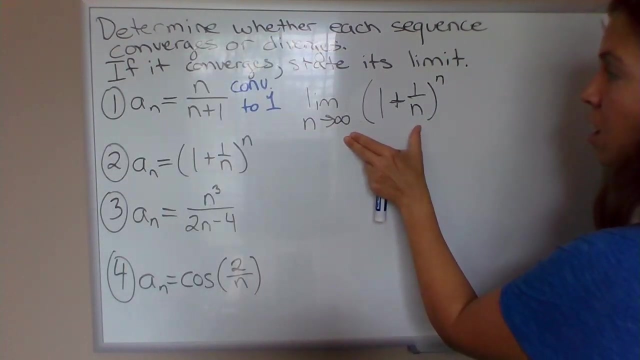 will. So example 2, we want to determine whether this sequence converges or diverges. So now we should take the limit of these terms: 1 plus 1 over n to the n, And this is a plus right here. So this is another nice limit to be able to just recognize. We did show back in section 5.6,. 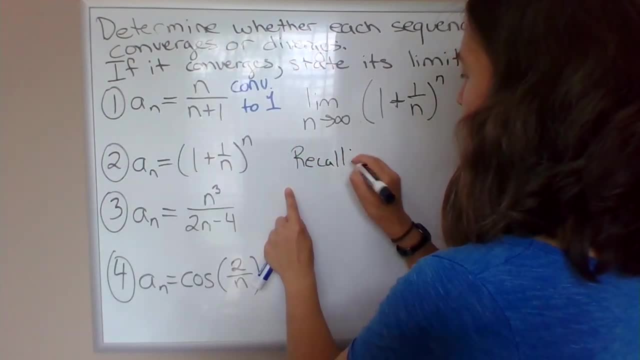 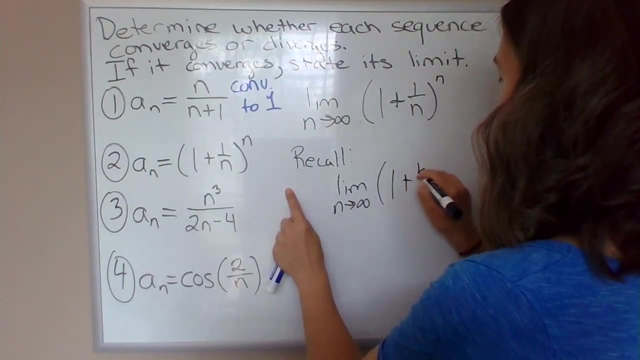 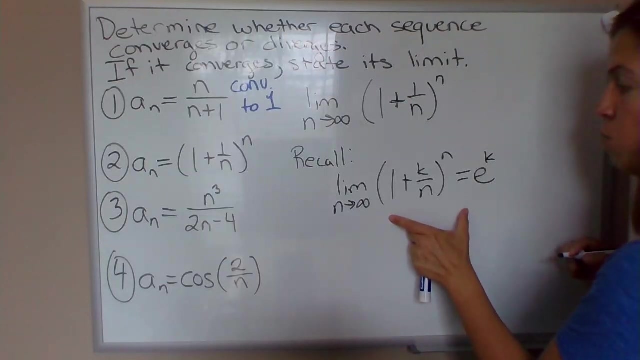 so I'll put a recall here that limits of this form, limit as n approaches infinity, of 1 plus k over n to the n is equal to e to the k. We did show this in section 5.6.. So 1 plus 1 over n to the. 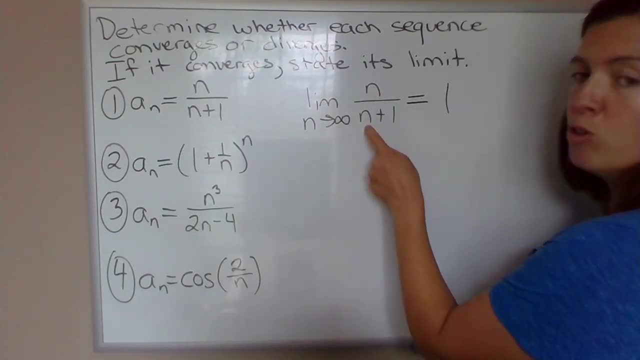 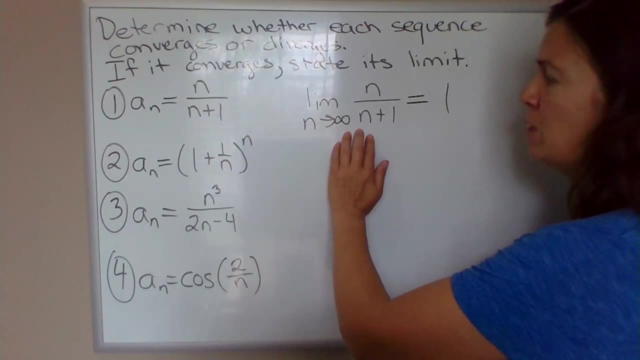 infinity over infinity. So you could take the derivative of the top and the derivative of the bottom, which would also give you 1 over 1.. But we're going to see limits of this form a lot, And so it's really best if you can recognize rational expression: same degree top and bottom. I just do. 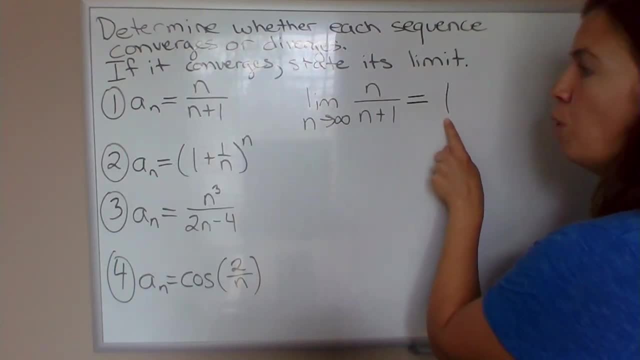 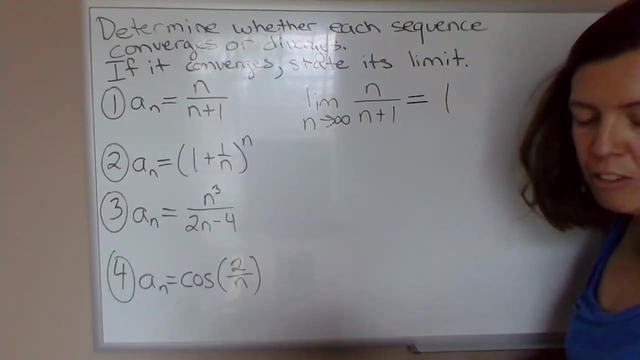 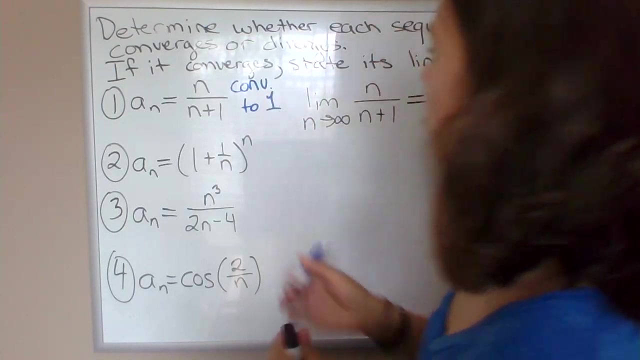 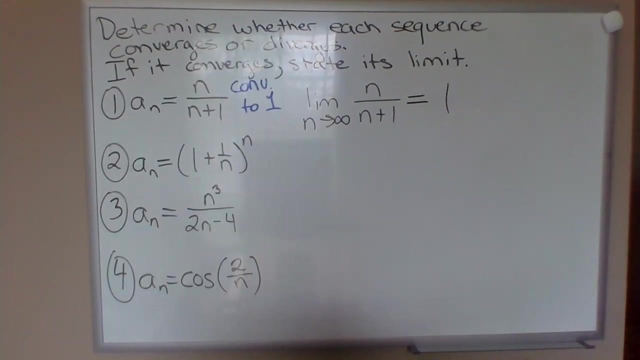 ratio of leading coefficients. It'll save you time. So when the limit is a finite number, as it is here, that means that the sequence converges to whatever that value is. So example 1 here converges to 1.. That's our answer, OK, And I'm going to erase. I won't erase yet, Actually I think I. 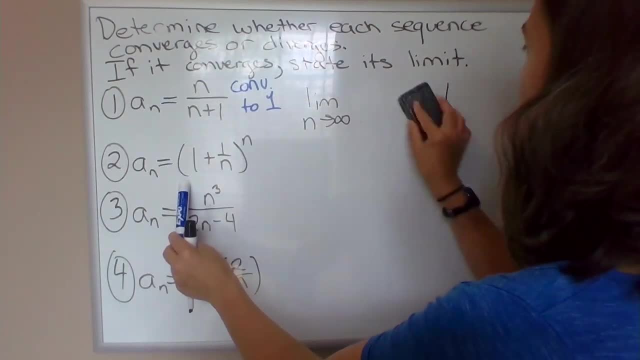 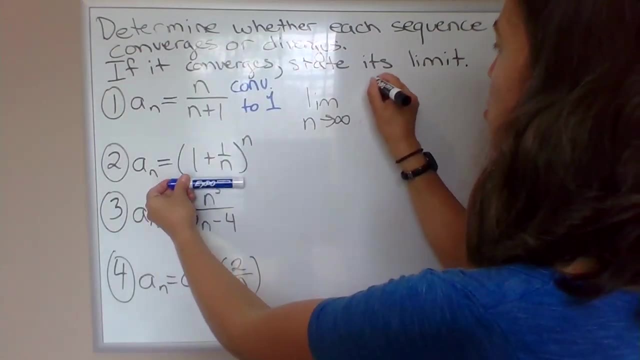 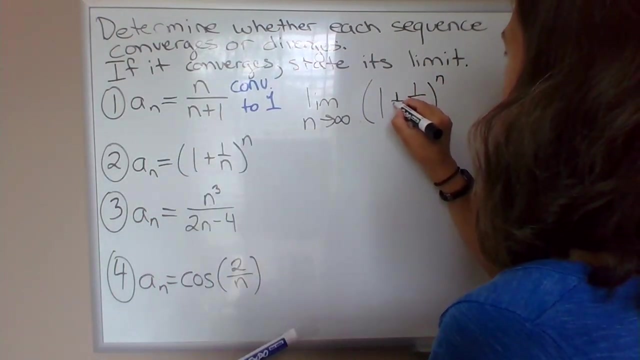 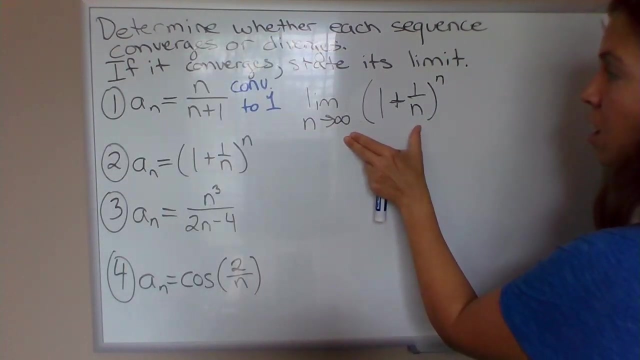 will. So example 2, we want to determine whether this sequence converges or diverges. So now we should take the limit of these terms: 1 plus 1 over n to the n, And this is a plus right here. So this is another nice limit to be able to just recognize. We did show back in section 5.6,. 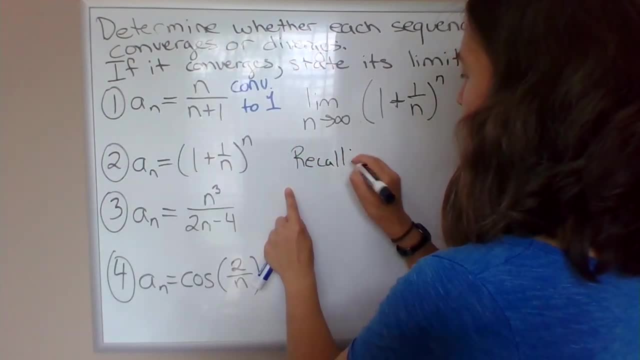 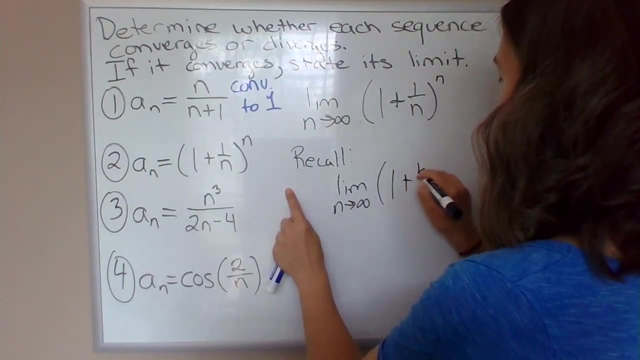 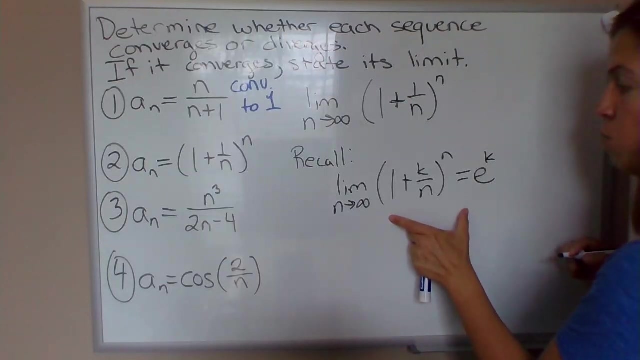 so I'll put a recall here that limits of this form, limit as n approaches infinity, of 1 plus k over n to the n is equal to e to the k. We did show this in section 5.6.. So 1 plus 1 over n to the. 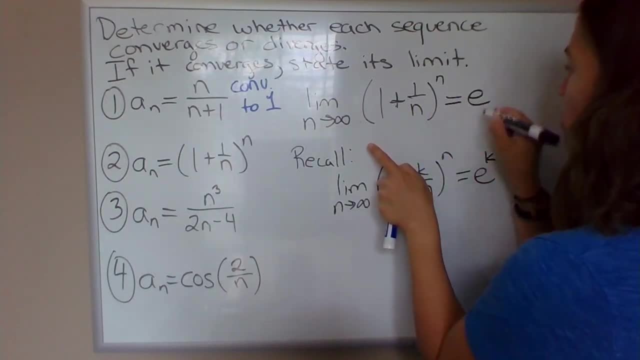 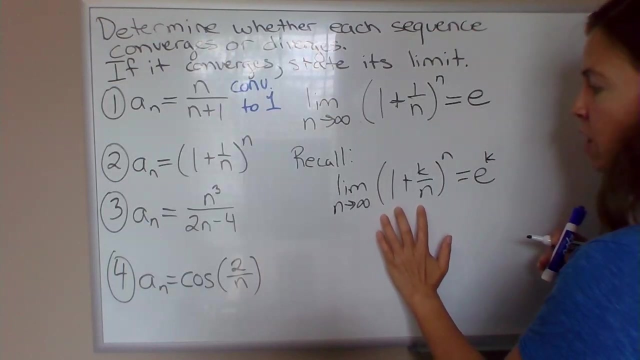 n. This is actually the definition of the irrational number, e, which is equal to about 2.7.. And then a lot of- I mean infinitely many- decimal places after that. But yeah, this is our definition of e. Or you can use, like I said, the work that we did in 5.6 to say, OK, well, it has. 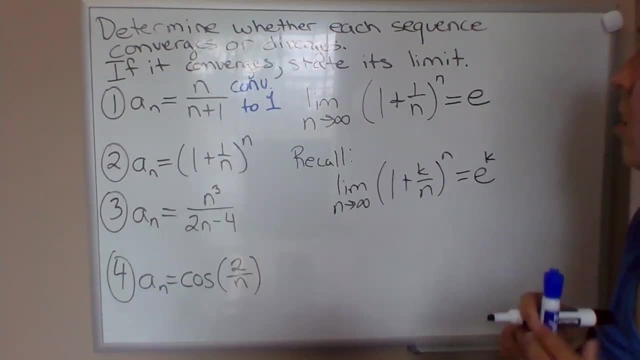 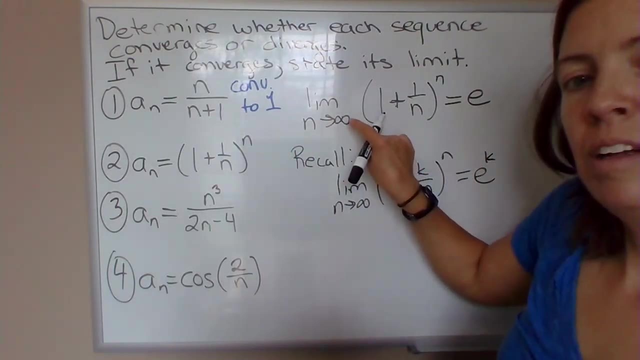 this form, so it's equal to e, to the first in this case. The other way to do this would be that whole deal where you take let l equal the limit, Take natural log of both sides, bring the exponent down, write it as a ratio and then apply. 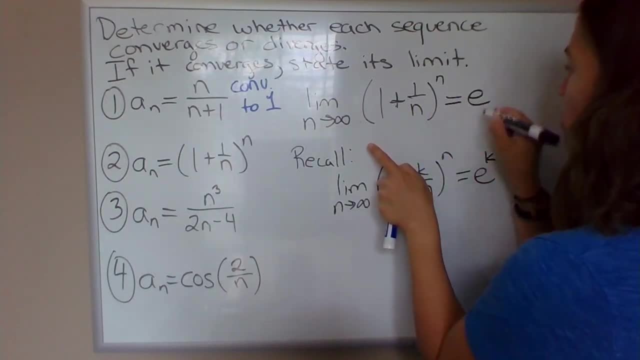 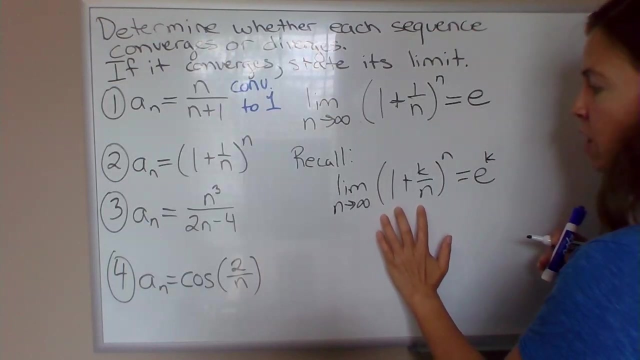 n. This is actually the definition of the irrational number, e, which is equal to about 2.7.. And then a lot of- I mean infinitely many- decimal places after that. But yeah, this is our definition of e. Or you can use, like I said, the work that we did in 5.6 to say, OK, well, it has. 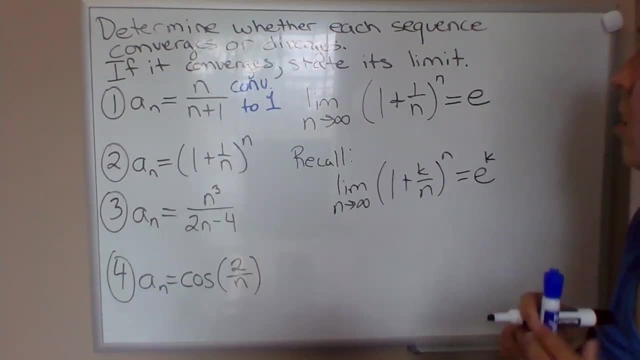 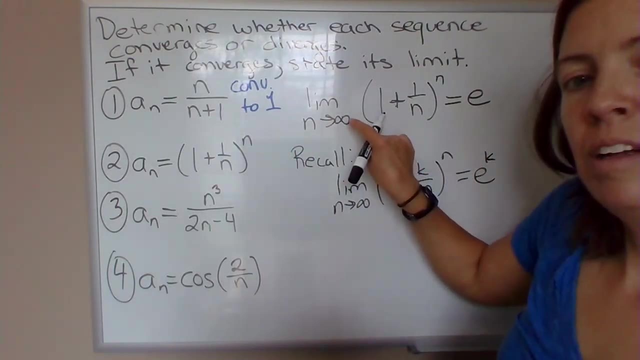 this form, so it's equal to e, to the first in this case. The other way to do this would be that whole deal where you take let l equal the limit, Take natural log of both sides, bring the exponent down, write it as a ratio and then apply. 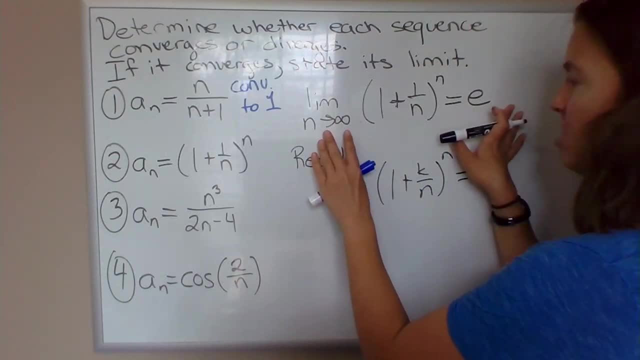 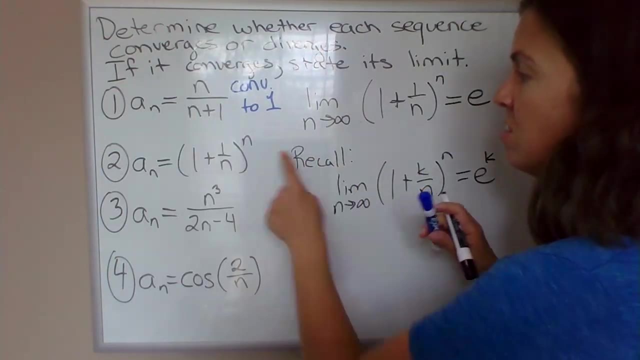 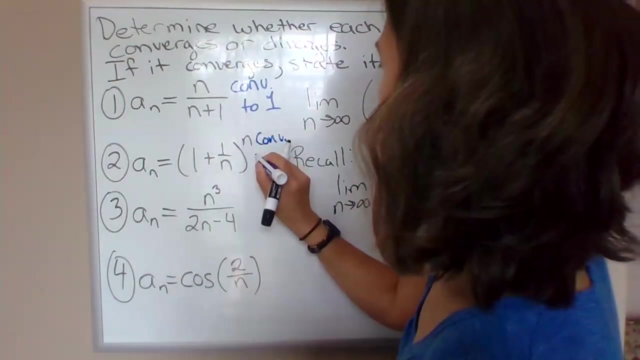 L'Hopital's rule. That's nice, But let's just leave it at that for the sake of this video. This limit is equal to e, to the first, which is a finite number, which means that this sequence right here converges to whatever that value is that the limit converges to. 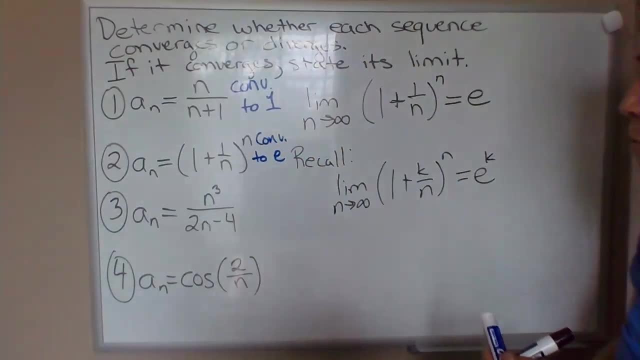 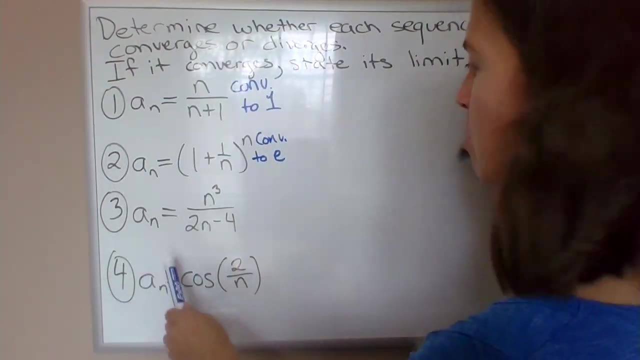 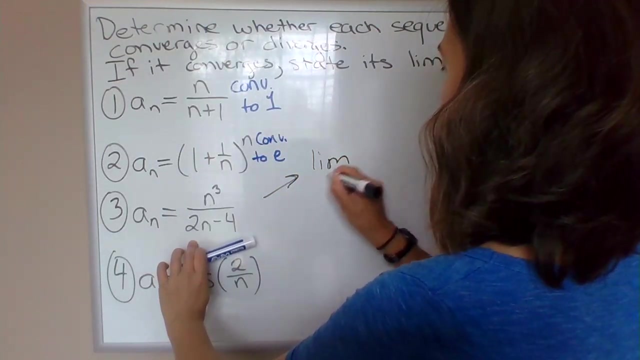 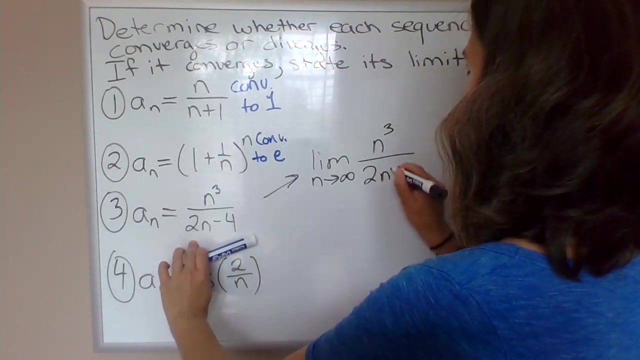 So in this case converges to e for number 2.. OK, Example 3.. So now we're working on this guy. So again, thanks to the sequence extension theorem, we can determine whether this sequence converges or diverges by taking this limit of n cubed over 2n minus 4.. 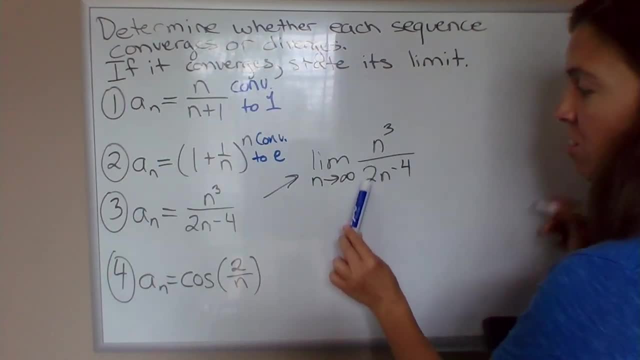 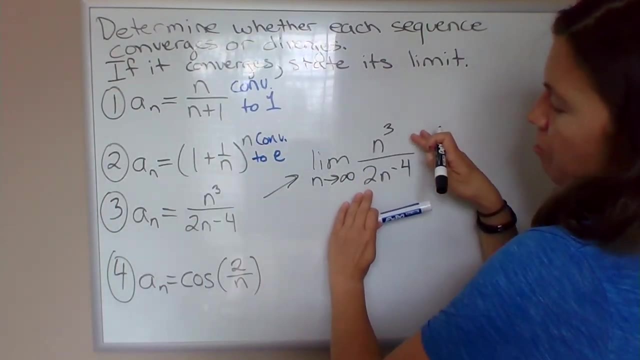 This has the form infinity over infinity, but it does not have same degree top and bottom. It has a higher degree in the numerator which might tell you something, But if you just think of it as OK, infinity over infinity, the degrees don't match. 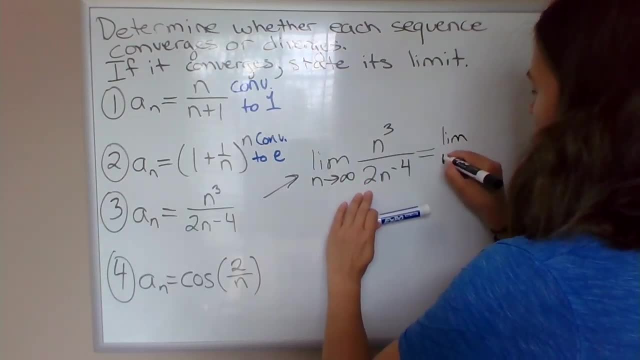 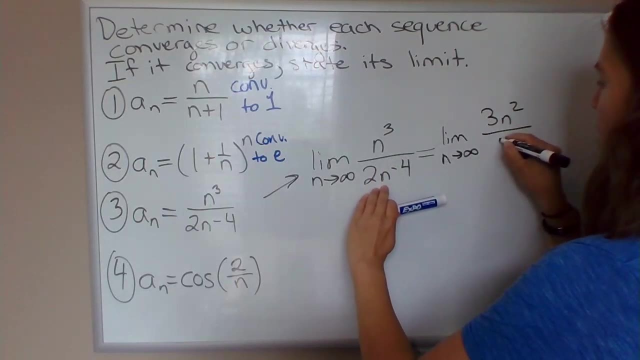 Let me apply L'Hopital's rule just to be sure. So limit, as n approaches infinity, of derivative of the top is 3n squared, Derivative of the bottom is just 2.. And so, as n approaches infinity, this is just 3 halves times infinity. 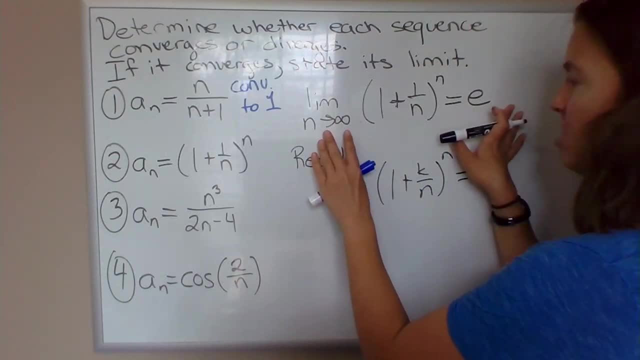 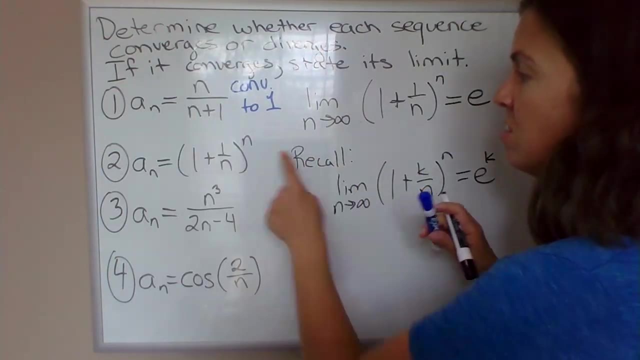 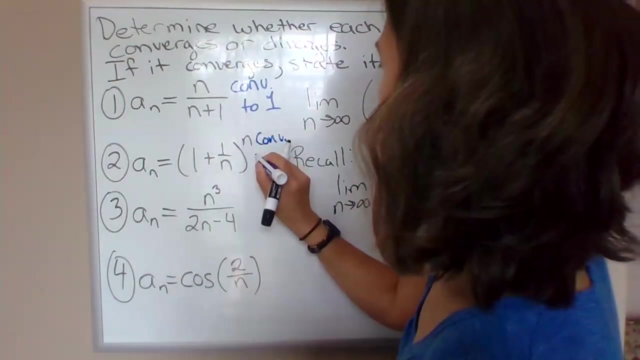 L'Hopital's rule. That's nice, But let's just leave it at that for the sake of this video. This limit is equal to e, to the first, which is a finite number, which means that this sequence right here converges to whatever that value is that the limit converges to. 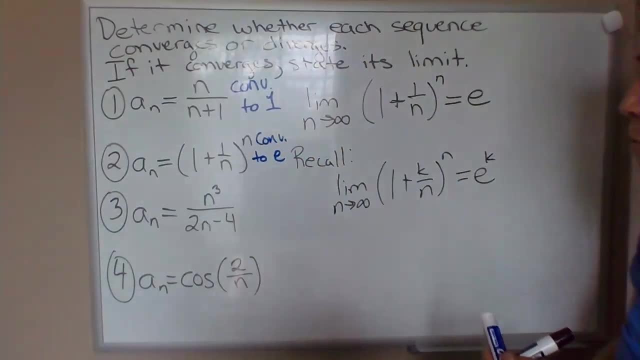 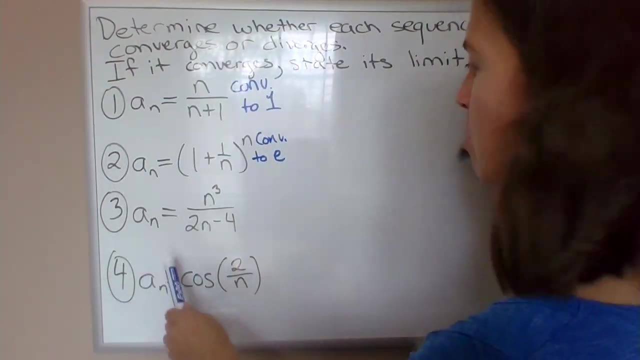 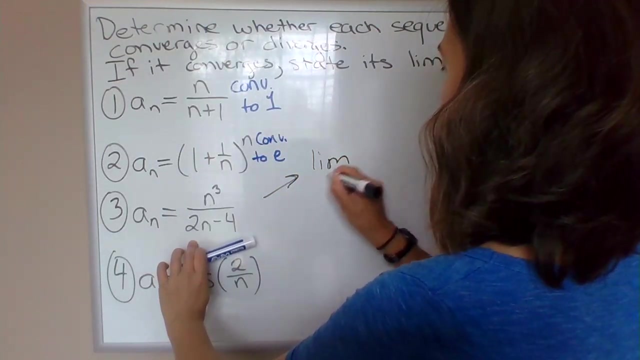 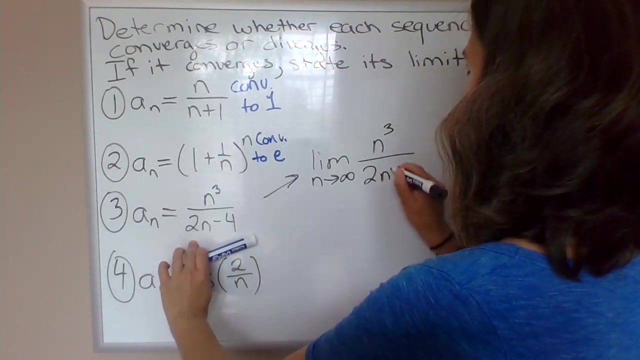 So in this case converges to e for number 2.. OK, Example 3.. So now we're working on this guy. So again, thanks to the sequence extension theorem, we can determine whether this sequence converges or diverges by taking this limit of n cubed over 2n minus 4.. 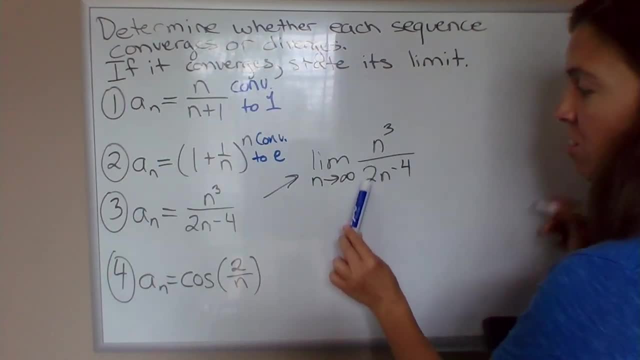 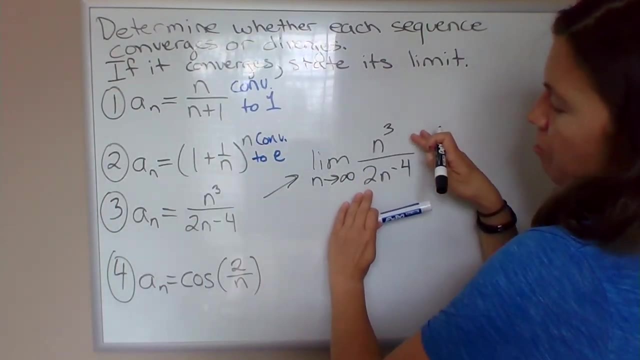 This has the form infinity over infinity, but it does not have same degree top and bottom. It has a higher degree in the numerator which might tell you something, But if you just think of it as OK, infinity over infinity, the degrees don't match. 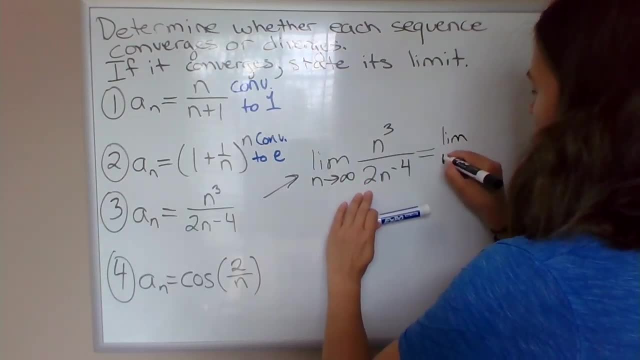 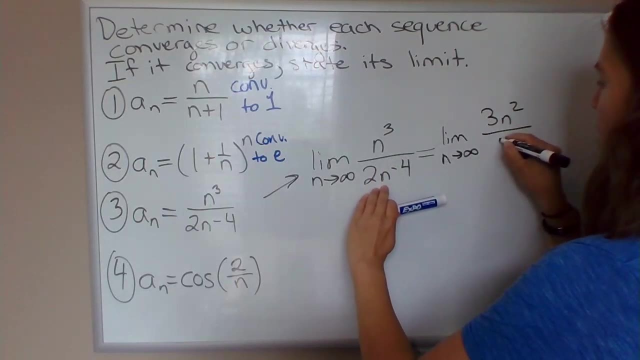 Let me apply L'Hopital's rule just to be sure. So limit, as n approaches infinity, of derivative of the top is 3n squared, Derivative of the bottom is just 2.. And so, as n approaches infinity, this is just 3 halves times infinity. 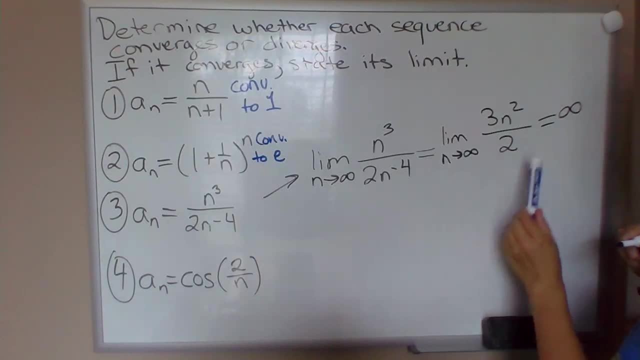 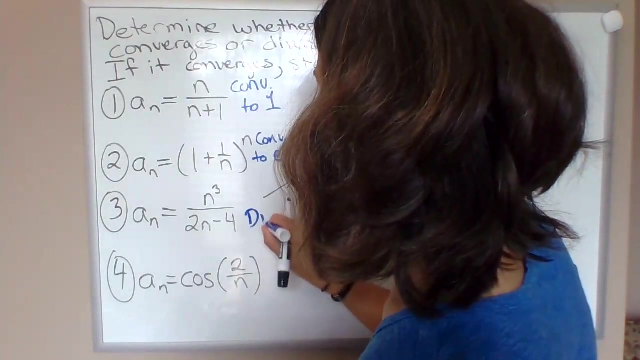 It's just increasing without bound. This is going to infinity. So remember, when a limit is equal to infinity, we're saying really that the limit doesn't exist. It's not approaching some finite number, It's just increasing without bound. So this limit diverges, which means this sequence: right here, number 3, diverges. 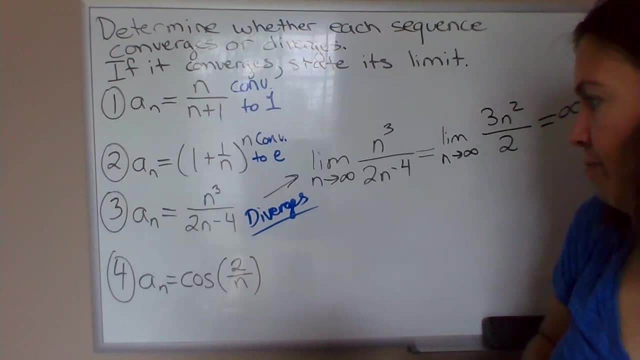 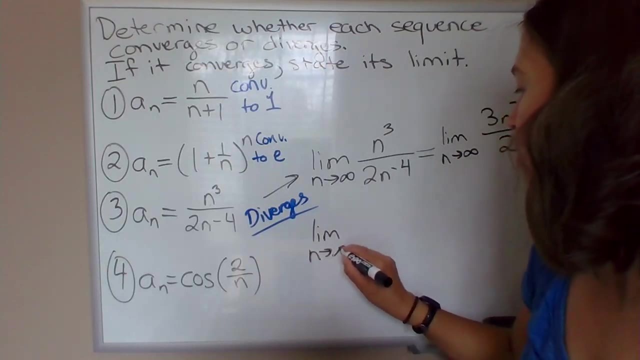 The limit of the terms does not approach some finite number. OK, last example, number 4 here, And I'm going to approach it exactly the same way. So this is how you determine whether a sequence converges or diverges, for the most part, 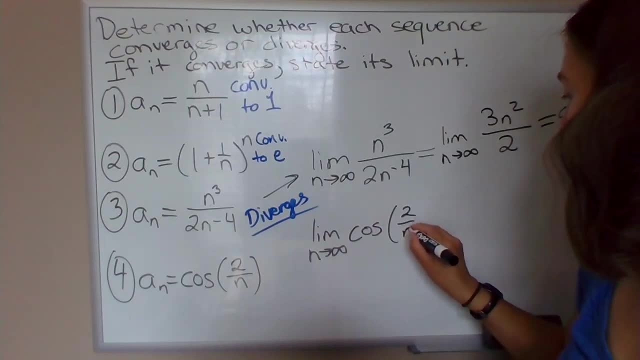 It's just take the limit of the terms. If the limit exists, it converges to that number. If the limit does not exist, then the sequence diverges. So in this case, cosine's a continuous function, So we're allowed to just move the limit inside here. 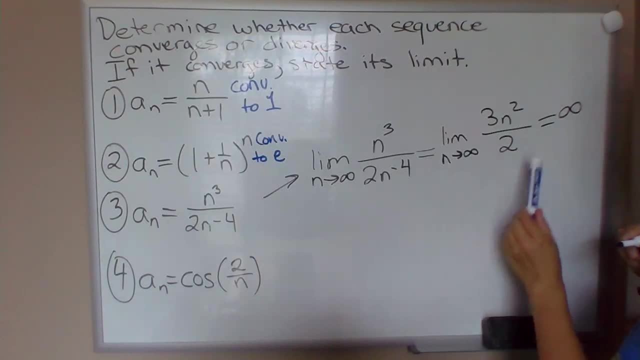 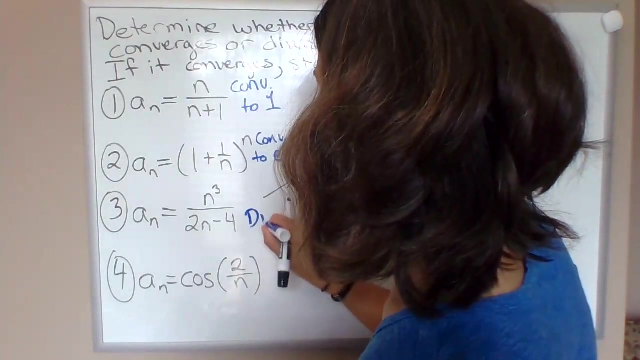 It's just increasing without bound. This is going to infinity. So remember, when a limit is equal to infinity, we're saying really that the limit doesn't exist. It's not approaching some finite number, It's just increasing without bound. So this limit diverges, which means this sequence: right here, number 3, diverges. 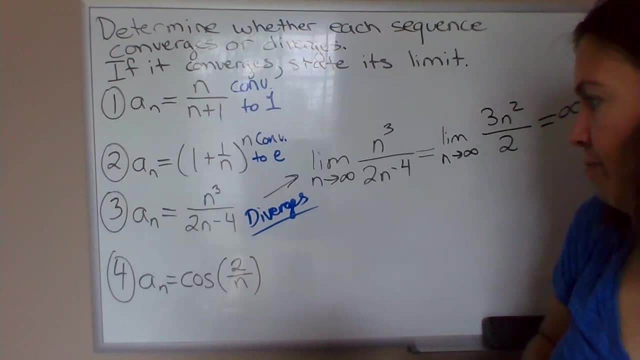 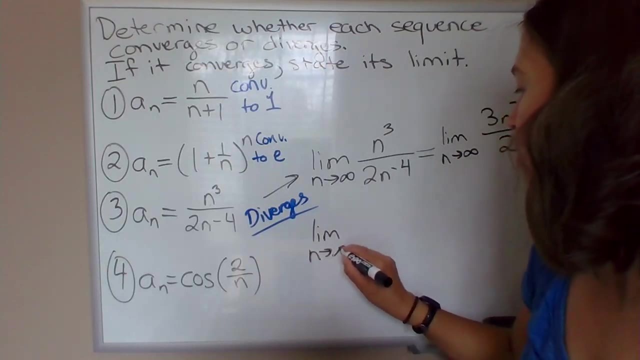 The limit of the terms does not approach some finite number. OK, last example, number 4 here, And I'm going to approach it exactly the same way. So this is how you determine whether a sequence converges or diverges, for the most part, 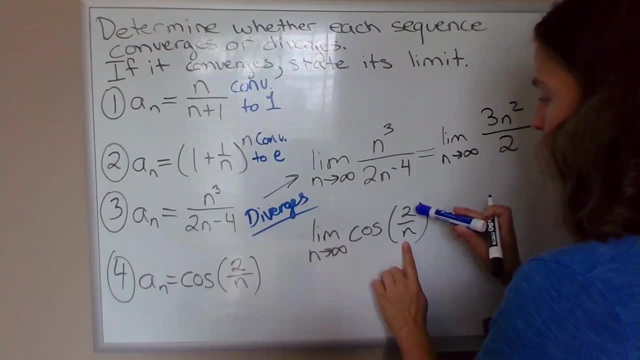 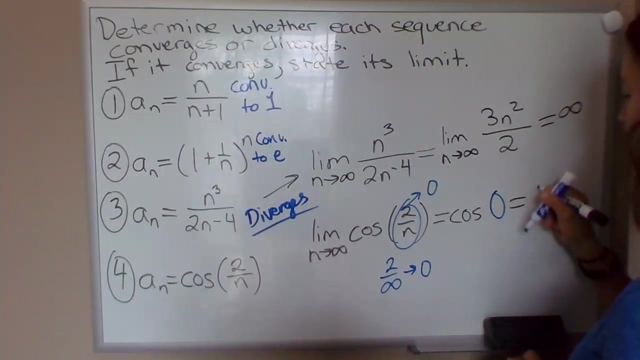 Take the limit, as n approaches infinity, of 2 over n. So that's 2 over infinity. So that's it's a finite number over infinity That's going to approach 0. So this right here approaches 0. And this is equal to cosine of 0,, which is 1..